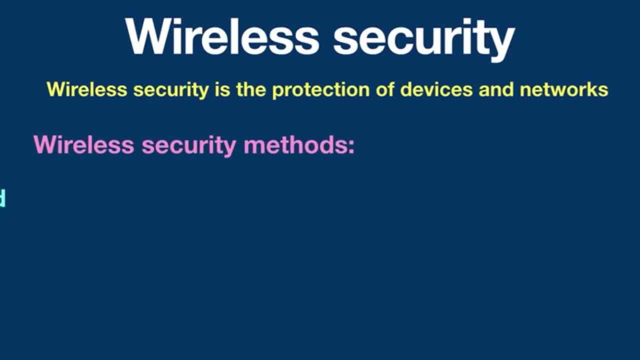 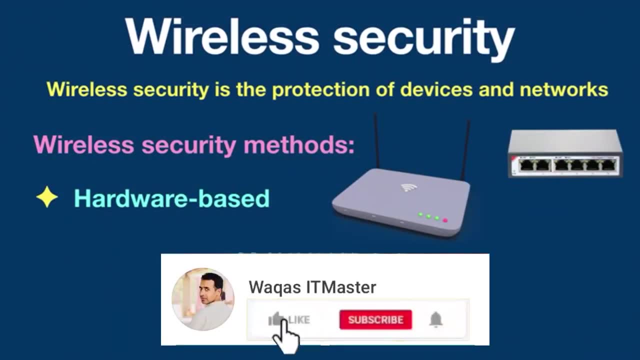 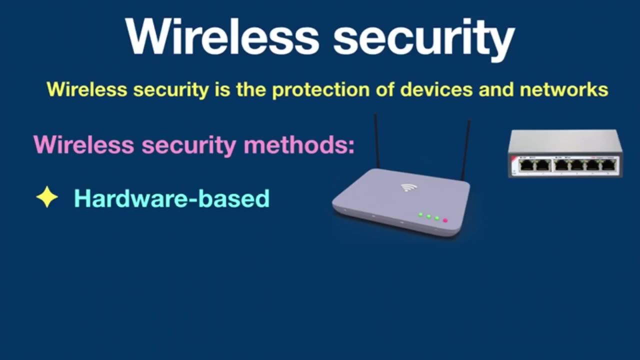 delivered through different ways, such as hardware-based. In this method, routers and switches are fabricated with encryption standards to secure all wireless communication. So in this case, even if the data gets compromised by cyber criminals, they will not be able to decrypt the data. Wireless setup of IDS and IPS: They help in detecting, alerting and preventing wireless. 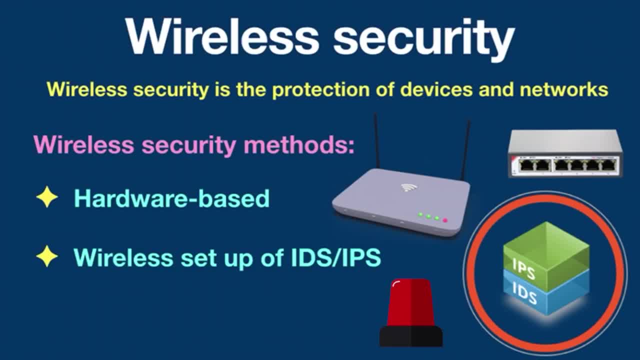 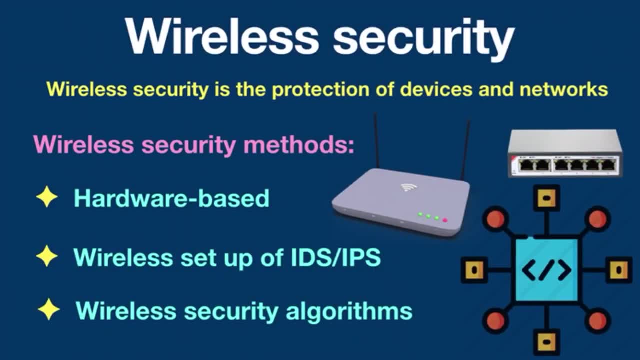 networks and send an alarm to the network administrator In case of any security breach. Wireless security algorithms such as WEP, WPA, WPA2 and WPA3.. They are also called Wi-Fi security protocols. These Wi-Fi security protocols not only prevent. 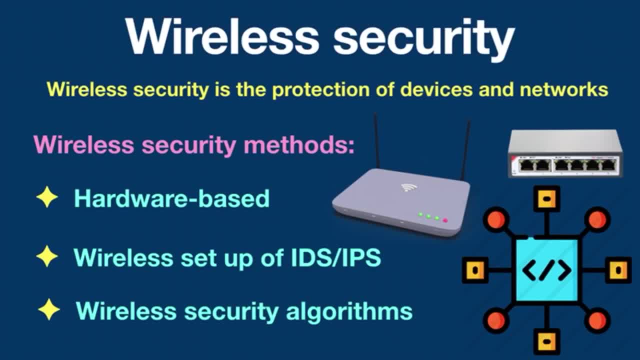 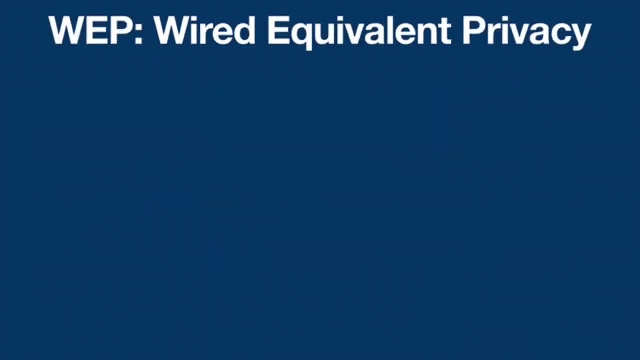 unwanted parties from connecting to wireless networks, but also encrypt private data sent over the airwaves. Let's have a closer look at these protocols. WEP- Wired Equivalent Privacy- is the oldest security algorithm, created in 1999.. It used initialization vector method to encrypt data. It provided the same security to wireless networks as it did for 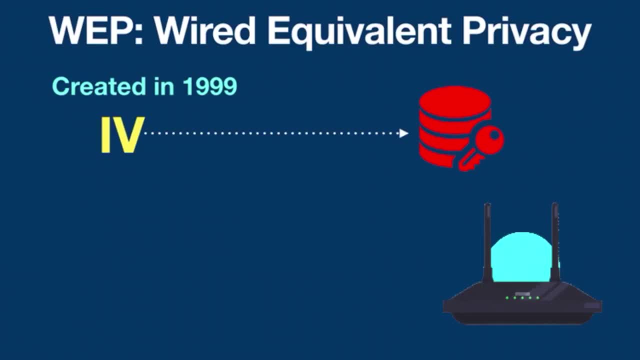 the wired network. The first versions of WEP algorithm were not predominantly strong enough, even when it got released, But the reason for this weak release was because of US limits on exporting WEP. After a couple of years, cyber security experts identified several swear flaws in WEP in 2001,. 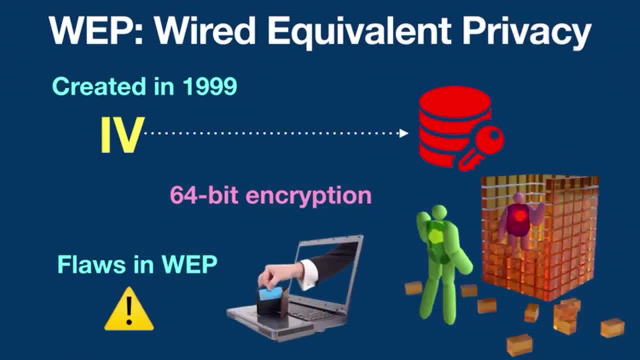 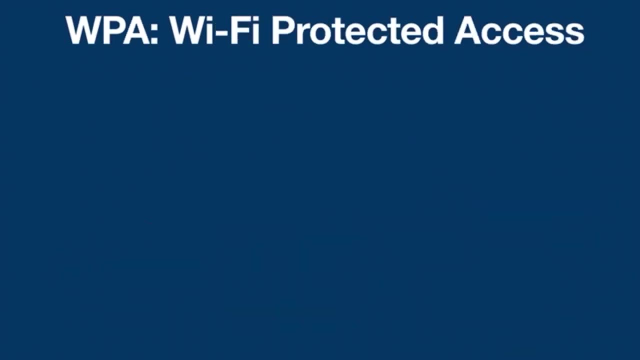 such as 64-bit encryption key, was vulnerable and insecure, so eventually leading to industry-wide security issues. To face out the use of WEP in both enterprise and consumer devices, And a new security protocol came in the market: WPA- Wi-Fi Protected Access is the next Wi-Fi alliance project that replaced WEP standards. 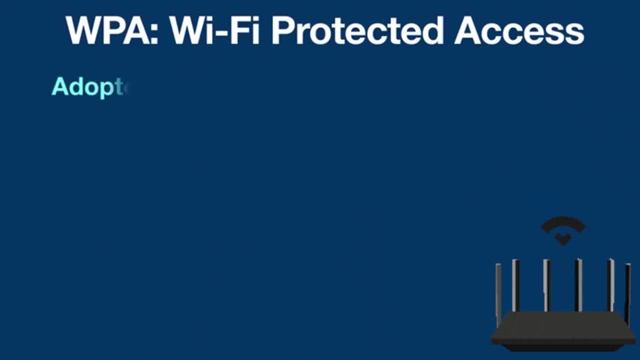 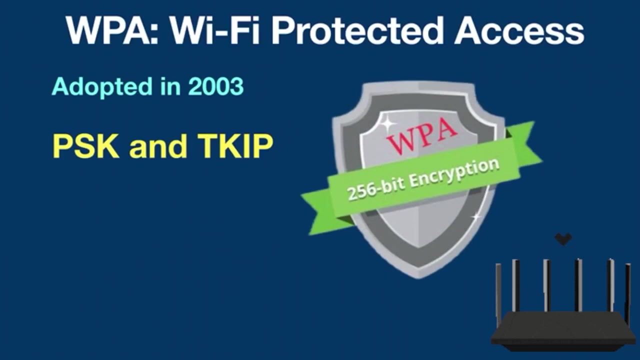 which had noticeable vulnerabilities. WPA was officially adopted in 2003,, one year before the retirement of WEP. WPA used pre-shared key and temporal key integrity protocol. for encryption. WPA used 256-bit encryption, which was a considerable enhancement above 64-bit key. Wi-Fi alliance. 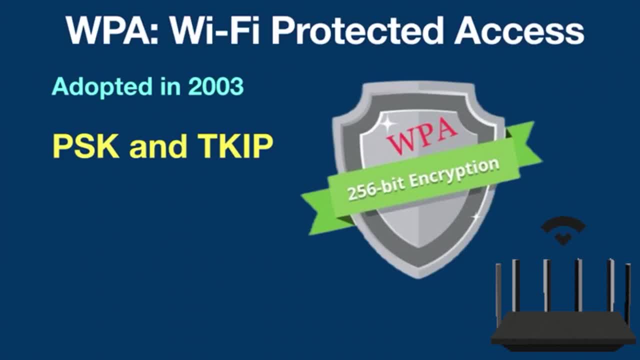 designed WPA to be backward compatible with WEP to encourage quick and easy adoption. Network security professionals were able to support the new standard on many web-based devices. WPA's use of WEPs was the most successful. This framework, however, provided the security, was not as comprehensive as it could have. 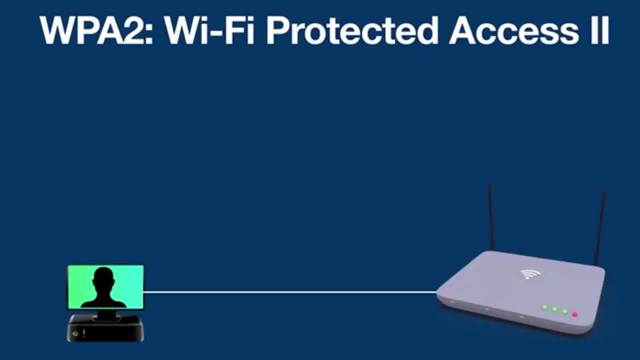 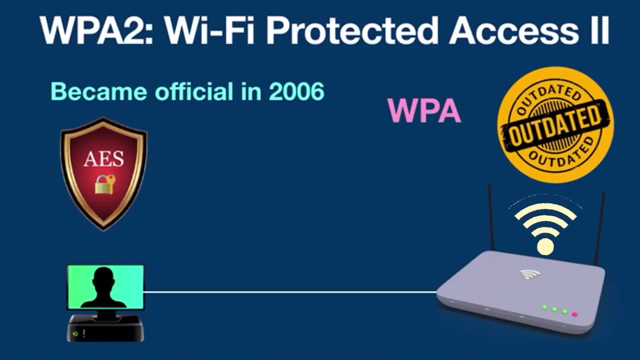 been So the new version came out- WPA2. It became official in 2006,. after WPA got outdated, It used advanced encryption standard algorithms as a necessary encryption component and counter-cypher mode Blockchaining message authentication capabilities. 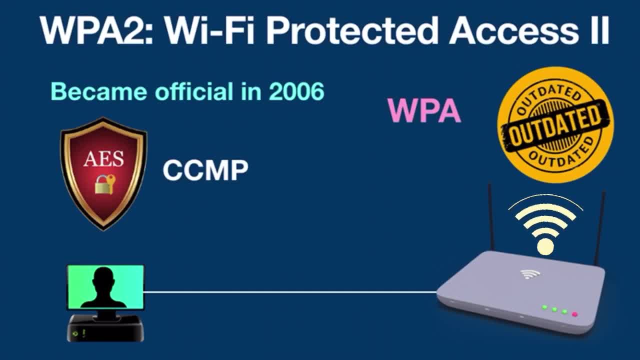 protocol by replacing TKIP. It was easier to configure and provided even greater network security than WPA1.. CCMP protected data confidentiality by allowing only authorized network users to receive data, as it used cipher block chaining message authentication protocol to ensure message integrity. WPA2 used a four-way handshake to authenticate the Wi-Fi client. It is a 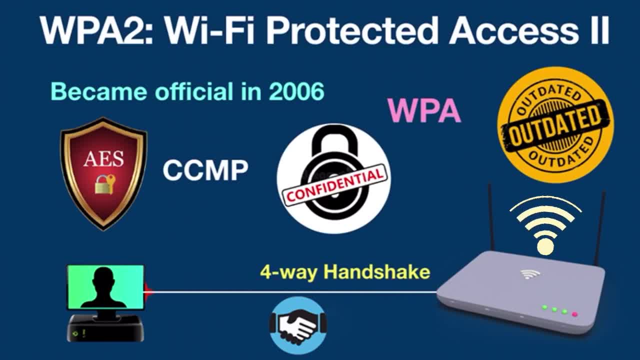 process of exchanging four messages between an access point and the client device to generate some encryption keys which can be used to encrypt actual data sent over a wireless network. In 2017, a security researcher found out a major security flaw in WPA2 key reinstallation attack vulnerability. 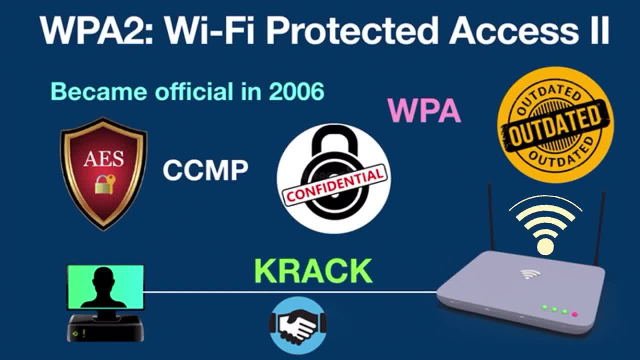 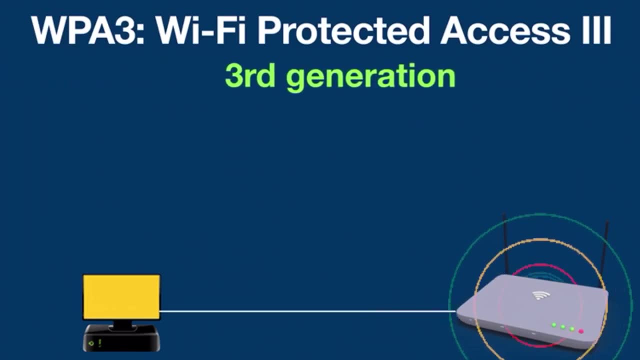 that exploited the reinstallation of wireless encryption keys. Crack vulnerability existed at the encryption stage and affected all WPA2 implementations. WPA3 is the latest and third generation of this family, developed under Wi-Fi alliance. It has personal and enterprise security support features. It uses 384-bit hashed message authentication mode: 256-bit. 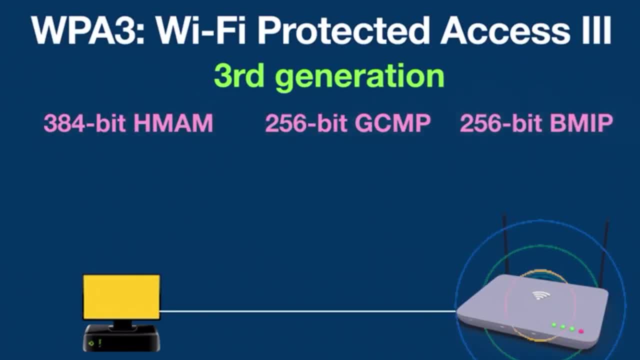 Glossy counter mode protocol and 256-bit broadcast multicast integrity protocol. WPA3 also provides perfect forward secrecy mechanism support. It is designed to deliver simpler configuration and even stronger encryption and security than any of its predecessors. It is also meant to work.